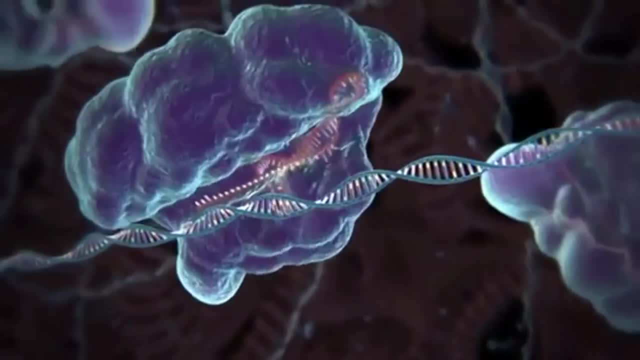 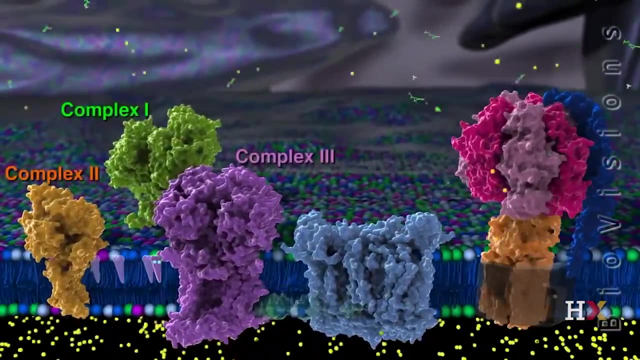 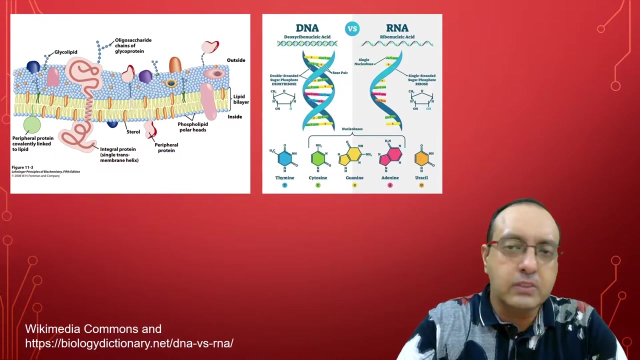 so today, let's discuss phosphorus cycle. now, phosphorus forms a very essential part of the biological organisms. for example, right from the start, if you consider the plasma membrane, it is made up of phospholipids, so phosphate is abundantly present in all the cells. 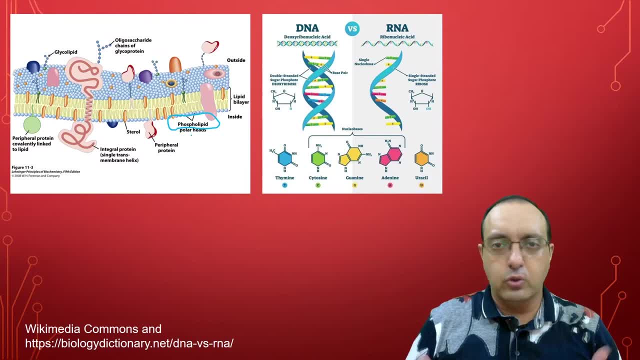 whether they are bacteria, whether they are, you know, protozoans, whether they are higher organisms. phospholipids: they form the integral part, almost 50-50 part, of the plasma membrane. so we need a lot of phosphorus if we want to create new cells. also, the genetic material of most living organisms know DNA, as well as 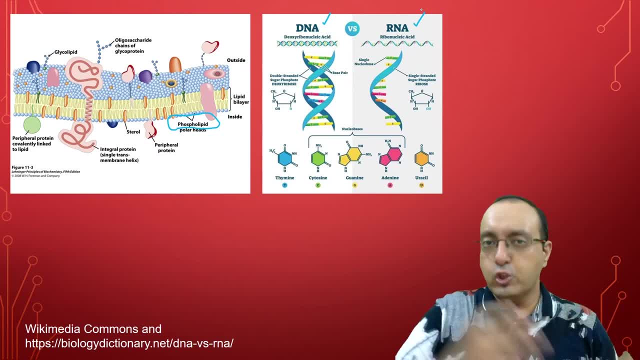 some living organisms, RNA. it also contains the sugar phosphorus back wound. so the phosphate is abundantly present in the form of PO 4 negative 3 in the form of sugar phosphate backbone. apart from that, there is a TP and other nucleotides which plaines, which play a very important 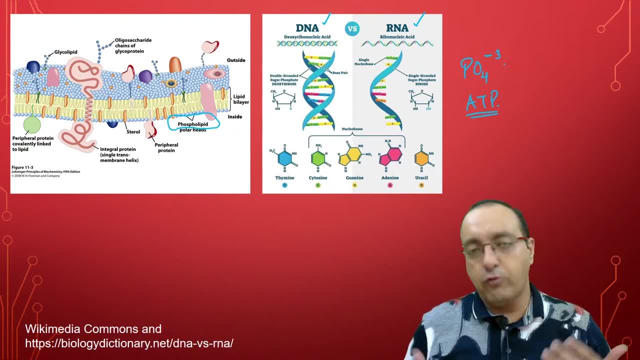 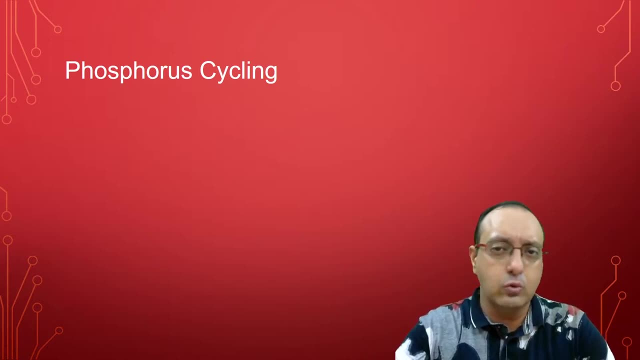 roles in energy transfer as well as in cell signaling. so phosphate is really really important for proper plant growth as well as for other the other organisms growth, so phosphorous cycling in the atmosphere and in the whole biosphere, takes place through basically four processes. the first is 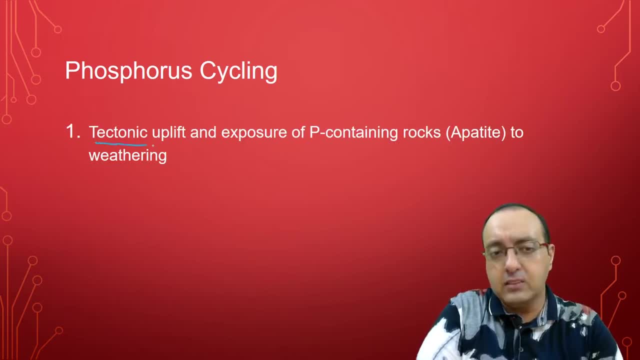 tectonic uplift. this is the rock based, you know, tectonic movements which basically expose rocks which are rich in phosphorus to weathering. weathering is the process by which rocks basically decompose, they release their mineral nutrients and then they are, you know, broken down. 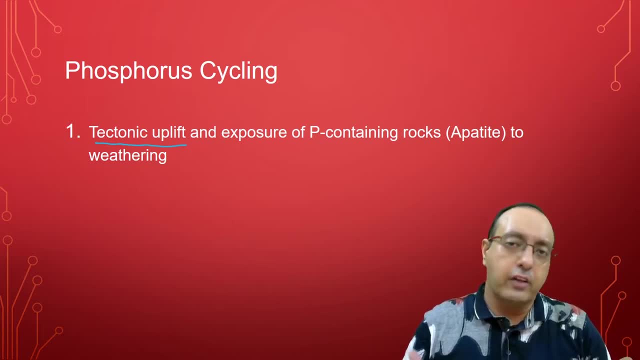 into smaller and smaller pieces as well, as well as to different different chemical compounds. the main phosphorus containing rock, from which most of the phosphorus in biosphere circulates, is called apatite. we'll look at its structure in more detail very soon. the second process is 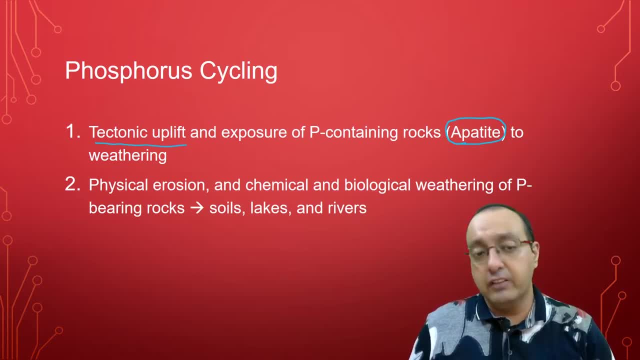 physical erosion, as well as chemical and biological weathering of phosphate bearing rocks- again apatite, for example- and this basically promotes the movement of phosphorus to soils, to lakes and to rivers. so again we have the tectonic uplift, which is the process by which rocks are produced. 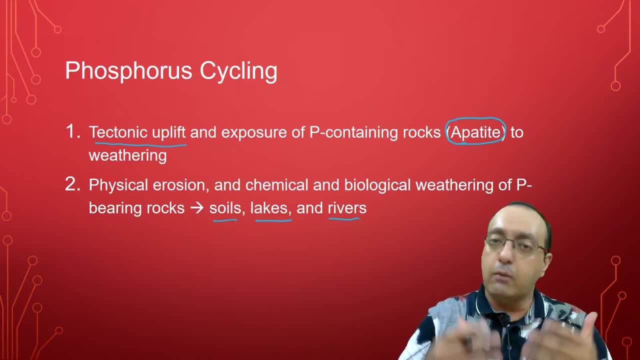 and then with the physical, chemical, biological weathering. many microbes are very good at weathering these rocks, so they release a lot of enzymes, they release a lot of acids which can degrade these rocks, which can lead to release of phosphorus into soils, lakes and rivers. that is the second process. 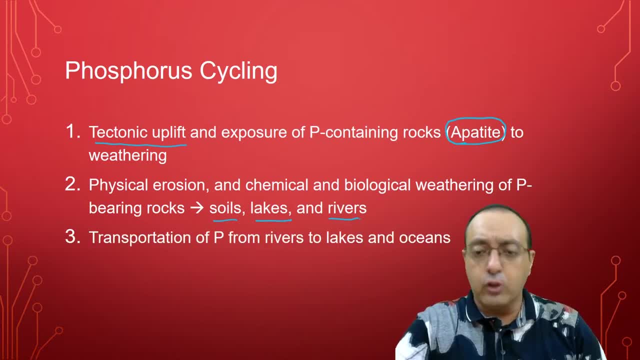 of phosphorus cycling. the third is transportation of phosphate from rivers all the way to lakes and oceans. so this is basically where the cycling is getting started. so this is basically where the cycling is getting complete. so you have transportation of phosphate from, you know, rivers to lakes and oceans and finally, we have the sedimentation of particulate phosphorus. 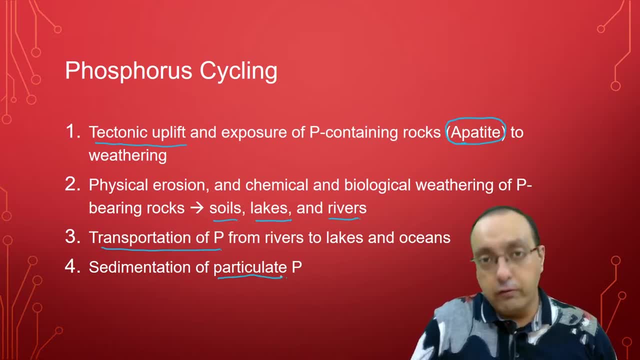 this is different from the, you know, the dissolved phosphorus, so there are various different types of phosphorus compounds available. particulate phosphorus is the phosphorus found in particulate, you know, small particles form and that is where it sediments and begins the formation of rocks. 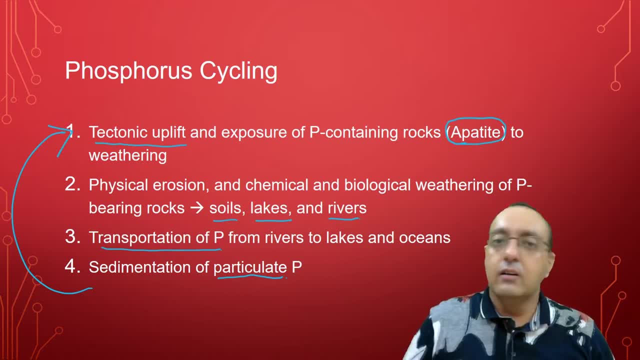 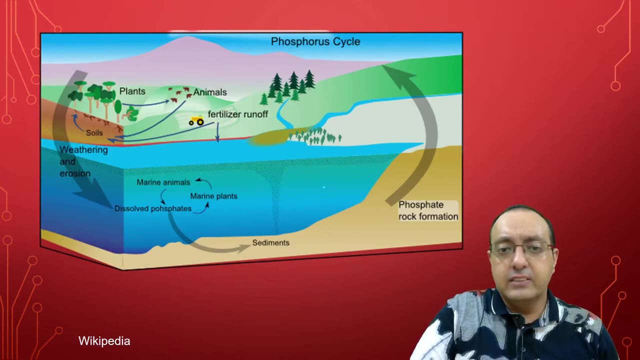 again. so it goes back to tectonic uplift and later exposure of these rocks, you know, once they come up to the surface again. so this is how the cycling goes on. so here is the phosphorus cycle in an image form you can see. for example, we have, you know, phosphate rock formation by the 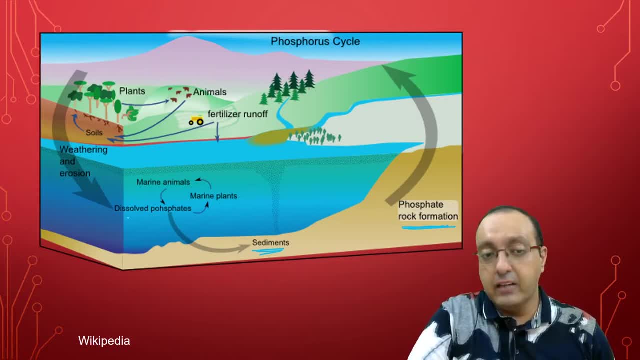 sediment buildup which was given by, you know, dissolved phosphates as well as the marine animals which were fixing a lot of phosphorus from немножко. so these are the Sachen, phosphate, so they form these sediments, they form these rocks later on, and due to the tectonic, 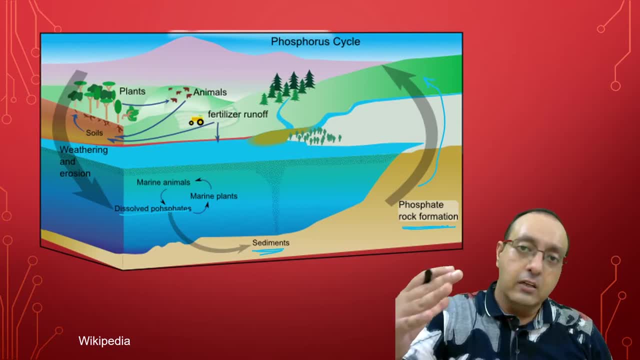 uplift and weathering of the rocks, it releases the phosphate to the environment, to the, you know, atmosphere, and then even through dust and you know, winds, these, for this phosphorus, you know, rains down on plants and animals, and plants and animals very much take up this phosphorus. 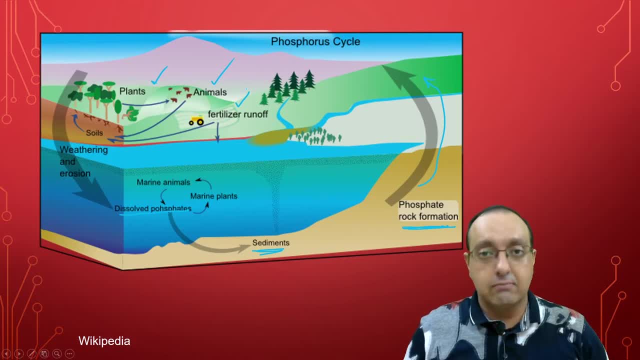 we also add phosphorus, which is causing a lot of problems. phosphorus and nitrogen: they make the- you know- water bodies very rich in nutrients and it leads to huge growth in algae, which is called algal bloom and later on. what happens in algal bloom is that when these algae die, the bacteria 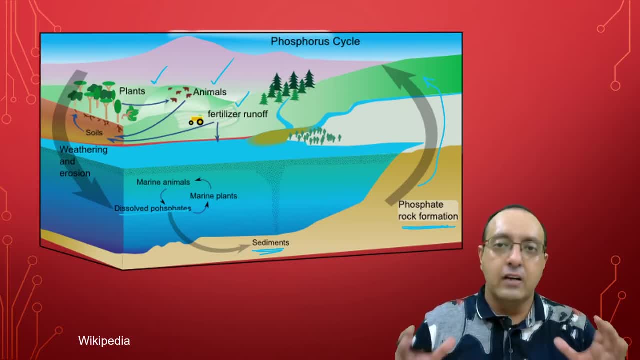 basically decompose their bodies and this leads to massive amounts of, you know, decrease in amount of oxygen available in these lakes and that leads to eutrophication and that leads to a lot of death of other organisms which are dependent upon dissolved oxygen. so that is a problem. so that is why soil farm runoff. 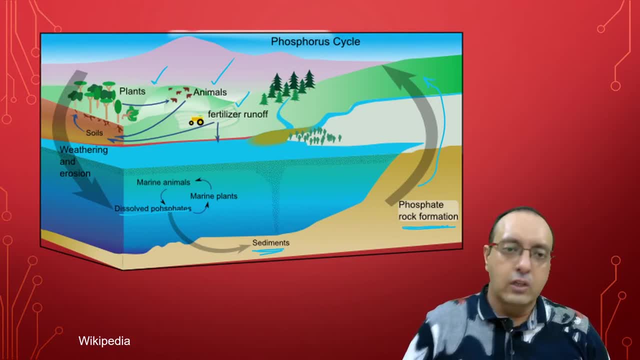 is a big problem- into the water bodies anyhow. so this is the weathering and erosion which brings the phosphate to the water bodies: oceans, lakes and rivers: sedimentation, phosphate rock formation and utilization here by physical, chemical and biological weathering, and this is the way that the phosphorus is discharging and then later up, later on, incorporation into 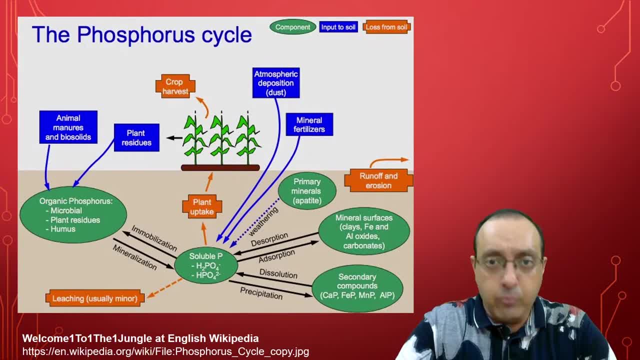 animals bodies. here is a little bit more closer look at phosphorous cycle in soil. so here we have different labels. the green label basically shows what kind of- you know- compounds and what kind of irons are present. the blue label shows how we get phosphorus into the soil and the orange label shows how we 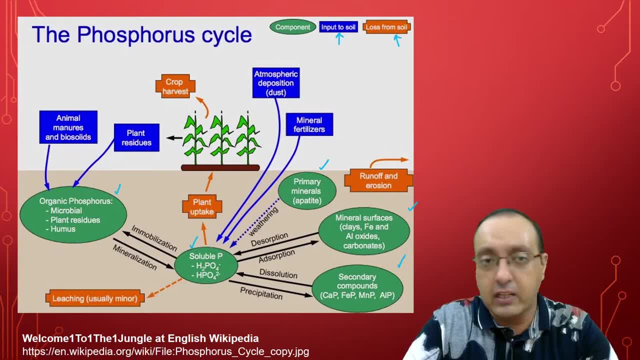 lose phosphorus from the soil. So let's take a look at the components. What are the phosphorus components? We have organic phosphorus in the form of microbial biomass, plant residues, humus, which is the decaying organic matter we talked about in our last video. 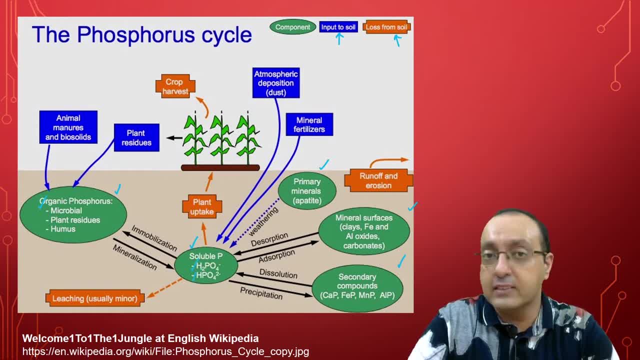 Soluble phosphate. you know these are H2PO4- and HPO4-2.. These are phosphate ions. We have mineral surfaces, so these contain clays, iron and aluminum oxides, carbonates, apatite. of course, this is the major phosphate-bearing rock. 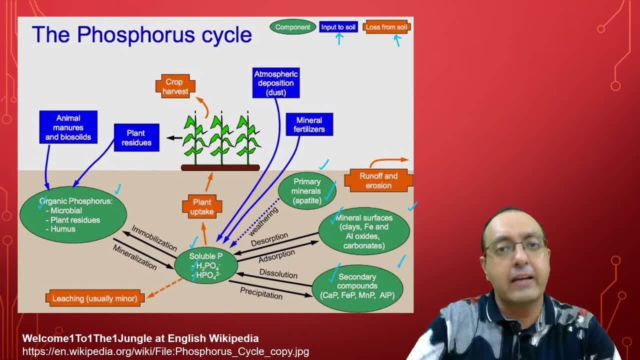 and secondary compounds, for example calcium phosphate, iron phosphate, manganese phosphate, aluminum phosphate. These are all phosphate-containing compounds present in the soil. How do we add phosphorus to the soil? We basically do it by four different methods: by adding animal manure or biosolids, by adding plant residues. 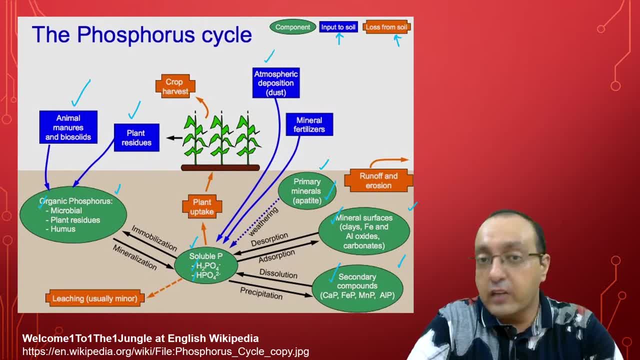 For example, manure. We have atmospheric deposition- the one that I talked about, the atmospheric weathering- and then phosphorus coming up as a dust, And we add mineral fertilizers in the form of phosphate compounds. So this is how we add phosphate to soil. 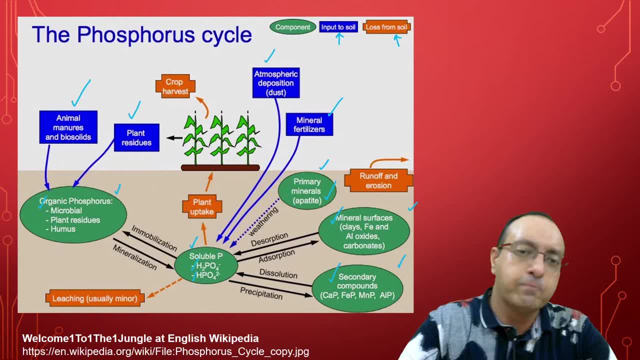 And how do we lose phosphate from the soil? We harvest our crops so that takes away all the phosphorus which has been incorporated into the- you know- cells of the crop that we are growing. We also have plants uptake this phosphate, phosphorus, so that is also lost from the soil, and then we harvest it. so that's a trouble. 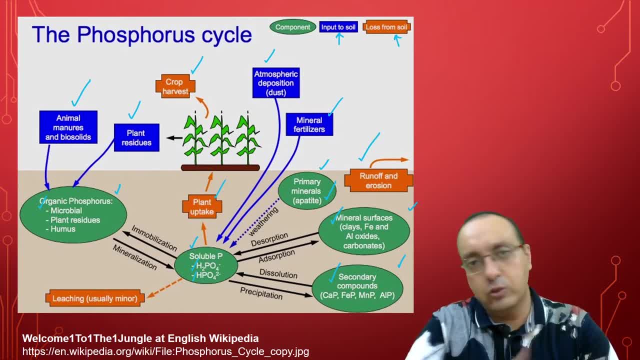 We also have runoff, you know, and erosion, so soil erosion due to running water bodies and that leads to leaching away of a lot of phosphorus And there is also minor leaching in, you know, in the soil. that is a little bit minor. issue majority it is the plant uptake and the runoff and erosion. 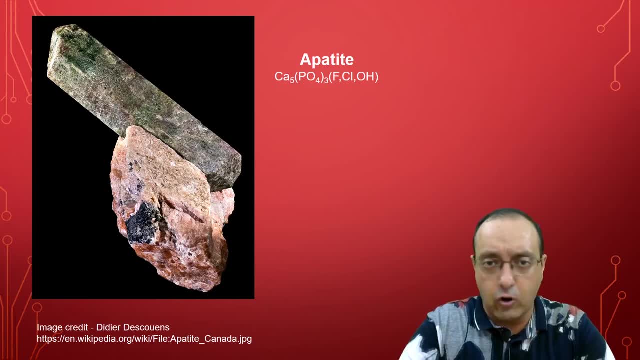 Here is the structure of apatite. this is a crystal from Canada. This is the common form of phosphate bearing rocks. Here is the formula: calcium 5,, PO4, 3, fluorine, chlorine and hydroxyl. So that is the basic, you know, reference unit of this crystal. 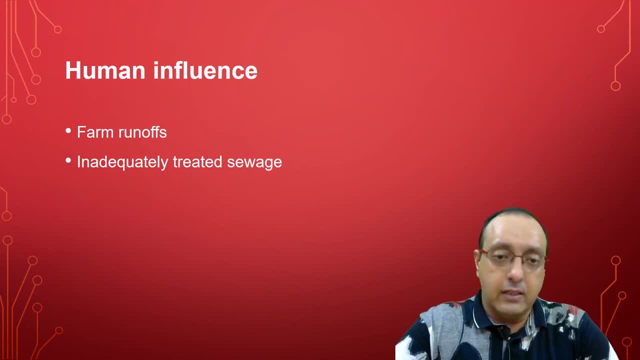 And human influence. I want to talk a little bit about it, especially from the regard of, you know, ecology as well as environmental concerns. Human influence in the form of farm runoff of phosphate is leading to eutrophication, as I already said. 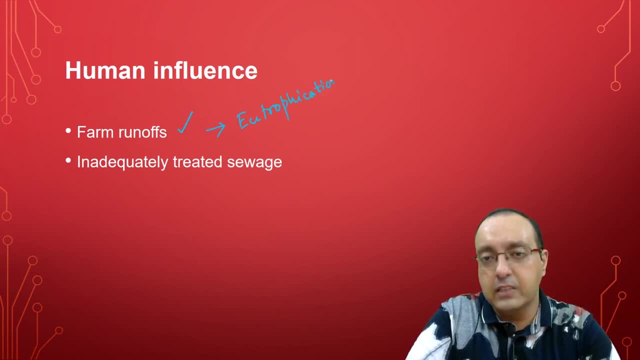 And this is lead to, you know, massive deaths of organisms in fresh water bodies, as well as in marine environments And inadequately treated sewage also. that is also a big cause of concern because it is not properly utilized by organisms, it is not properly broken down by organisms. 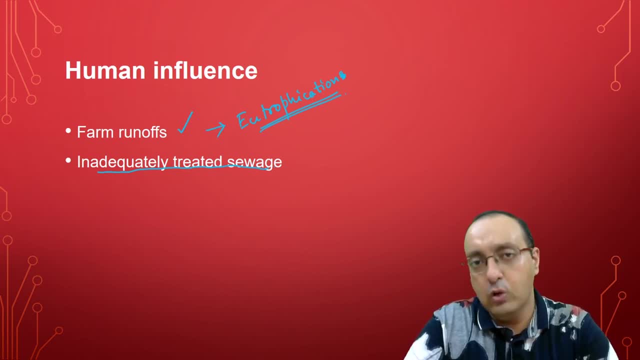 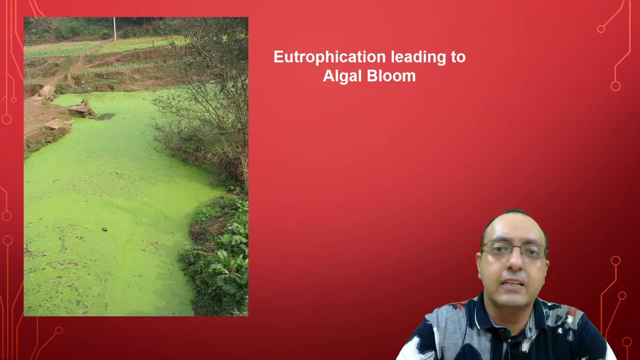 And that causes a lot of problem when we release it into Water bodies. okay, Here is the picture. it's a familiar sight. I think you must have seen it in villages also. This is basically a human caused activity. This is eutrophication leading to this massive bloom in algae. 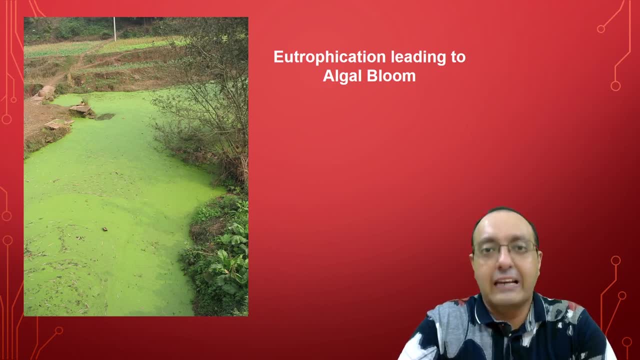 This is not a problem. this is actually just growth of algae. But the problem will be when bacteria will eat these dead algae, when they will die, And then they will, you know, get rid of a lot of oxygen. They will use up a lot of oxygen, which is